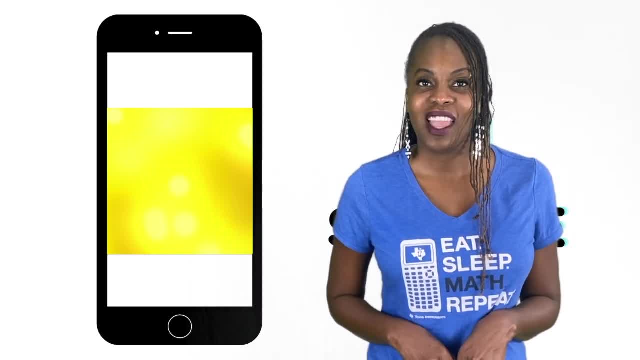 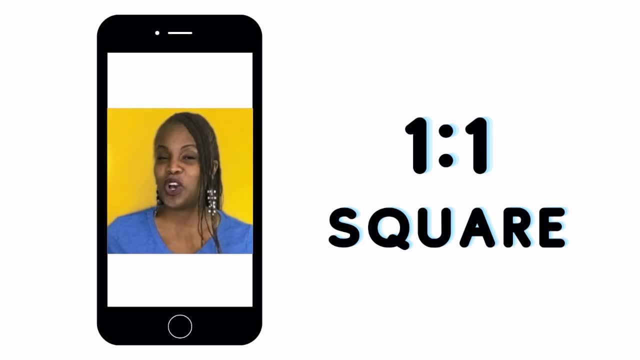 or your pictures in a nice little square frame. in fact, hold on a second. you see, here I am in my cell phone with a 1 to 1 ratio. it's a square ratio, 1 to 1. you might not have realized it. it's called an aspect ratio because it's how you're. 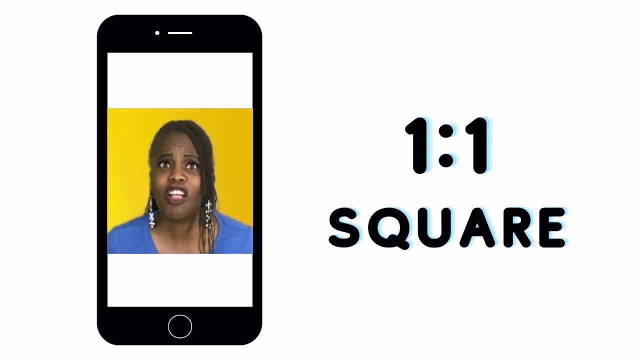 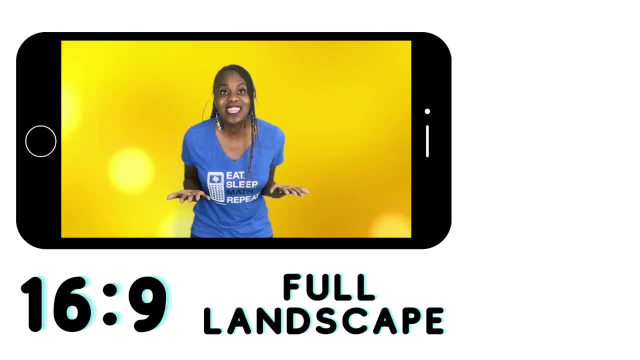 viewing your video or your pictures, and we use it all the time, or maybe you use a ratio like this, so check out this. this is a landscape ratio. it's wider a 16 by 9, and this ratio is in lowest terms because there's not a factor that 16 and 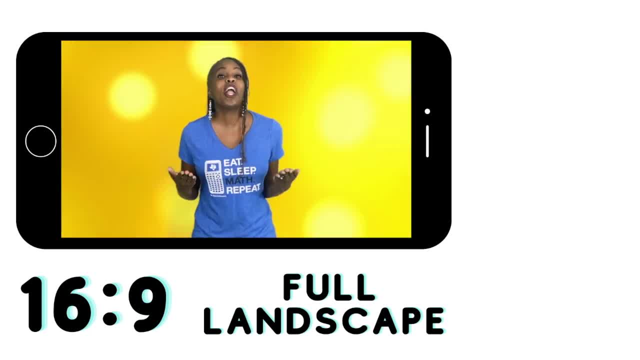 9 have in common. most videographers want you to film in this ratio if you're using your cell phone, like I am right now. see, so you guys use ratios all the time. let's think of different ways we might use ratios that don't involve cell phones. what about cooking? oh my goodness, there are so many. 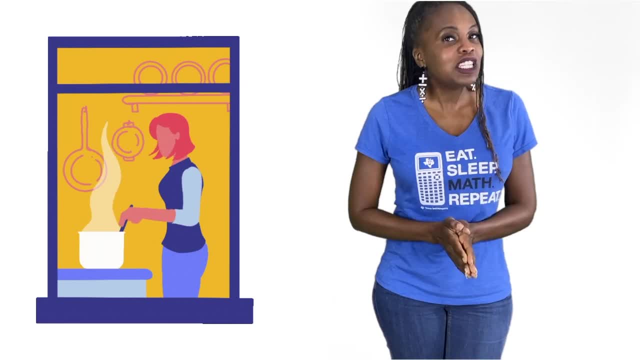 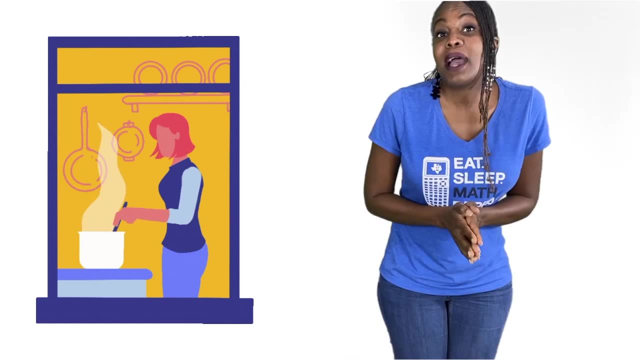 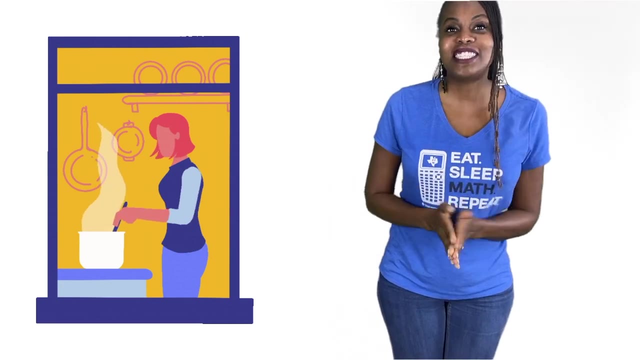 different ratios when you're cooking a meal, especially when you think about the recipes, it might call for one part this and one part that. it might ask you if you want to divide things up and give this portion of a meal to these portion of people. for example, I love ordering pizza right or even cooking pizza, and I 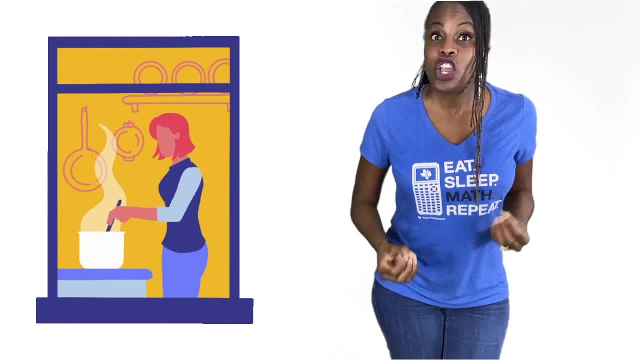 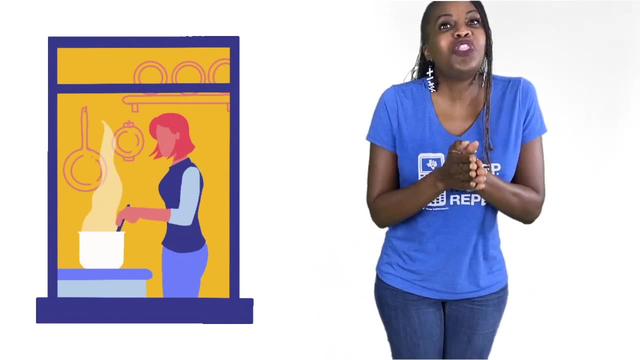 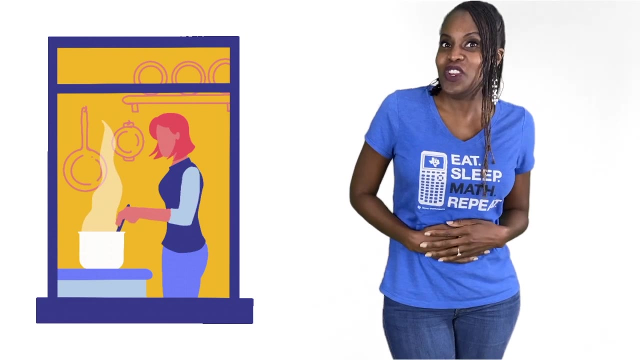 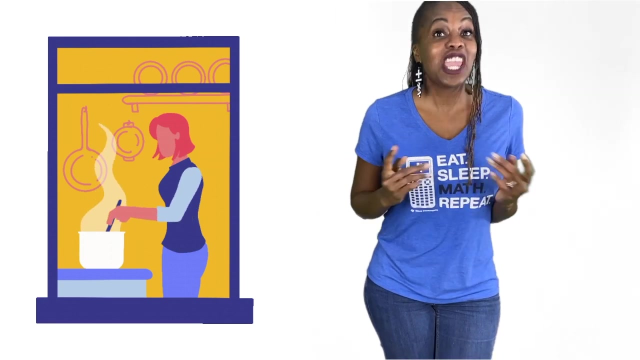 always have to figure out how many slices could I give each person, so that way every part of the pizza gets distributed equally. so those are great examples of ratios that you see all the time, especially if you're like me and you like pizza. in fact, I wonder what she's cooking. I'm getting kind of hungry. here's another. 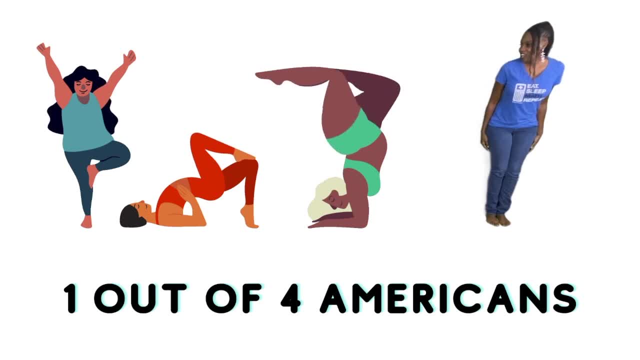 example. oh, I guess we're working out. have you ever tried yoga? well, if you have, you fit this ratio, because one out of four Americans have tried yoga in their life. this is another example of ratios. in fact, these type of ratios, these type of one and four, or